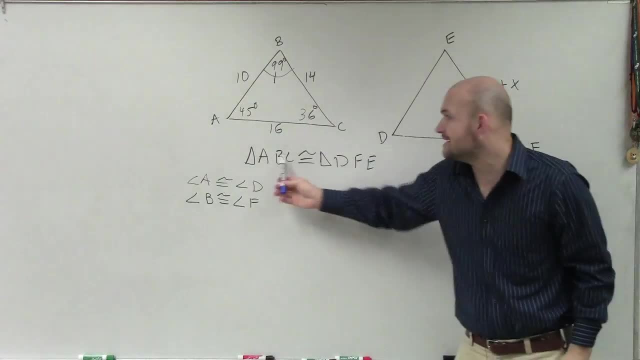 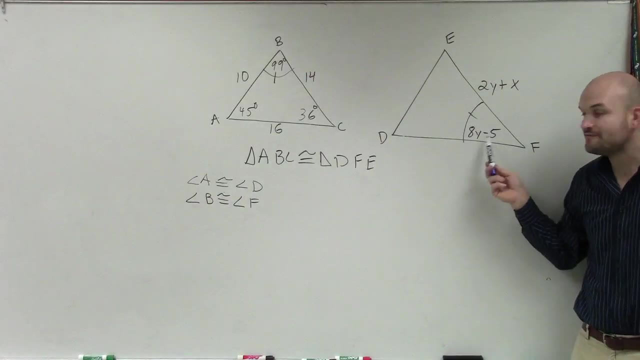 e has to be equal to b. No, that's not what the directions say. They say b is congruent to f. That means these two angles are equal in measure. all right, So if I want to figure out what y is, don't set this equation equal to. 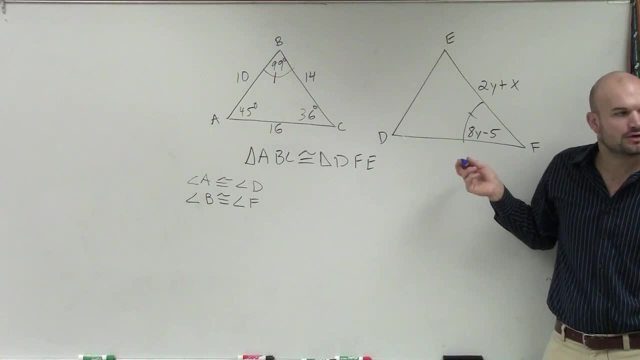 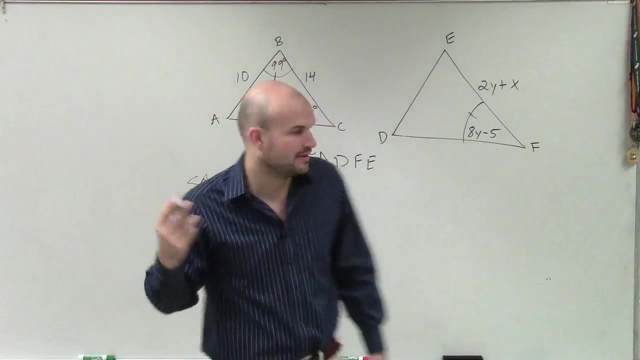 36, because they're both in the right-hand lower corner of the triangles. Does everybody see what the change is on this problem? Blake got that Okay, So therefore now I can set up an equation to solve for y. I can say: 8y minus 5 equals 9y. 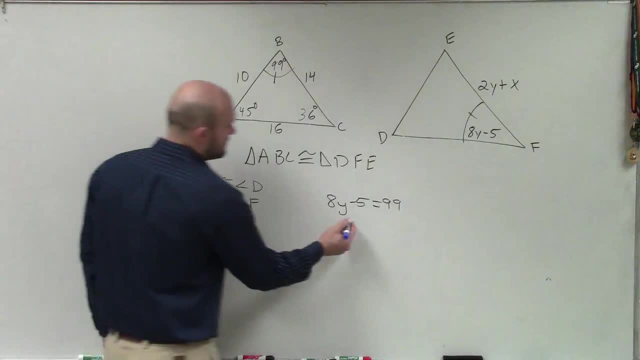 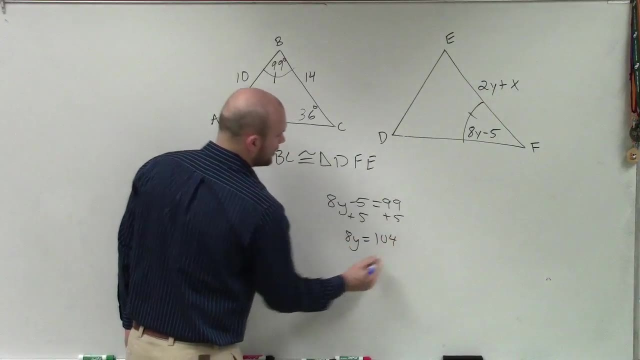 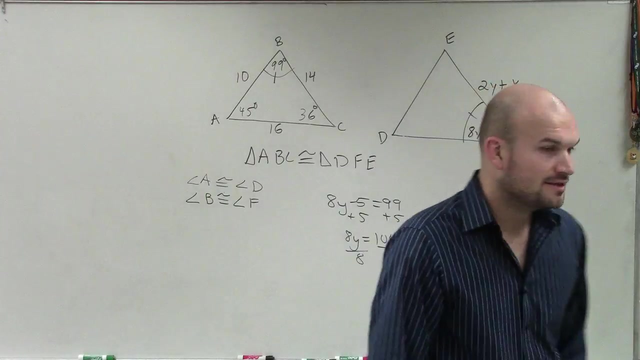 I'll add up this. so I've got y equals 99. So now I add 5.. I have 8y equals 104, divided by 8, divided by 8. We know that 8 goes into 80 10 times, leaving me with a remainder of 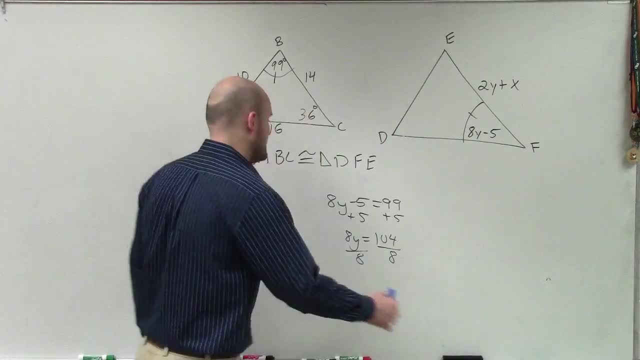 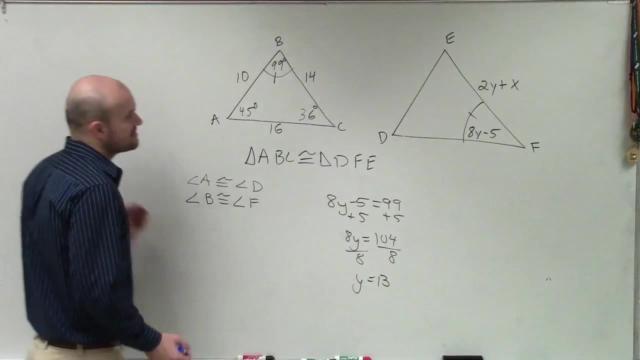 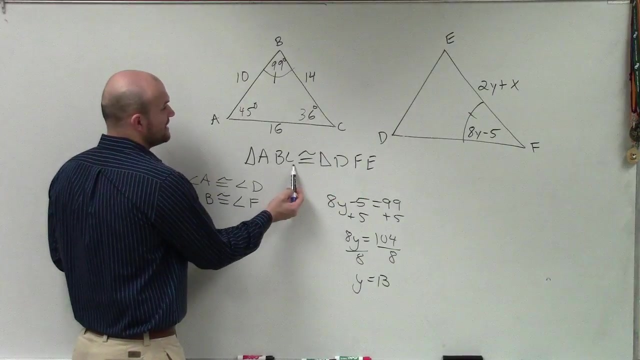 24.. 8 goes into 24 3 times, so therefore y equals 13,. all right, Now to find the value of x. we know that…. Now let's go and look at this. So Fe is congruent to Bc. OK, 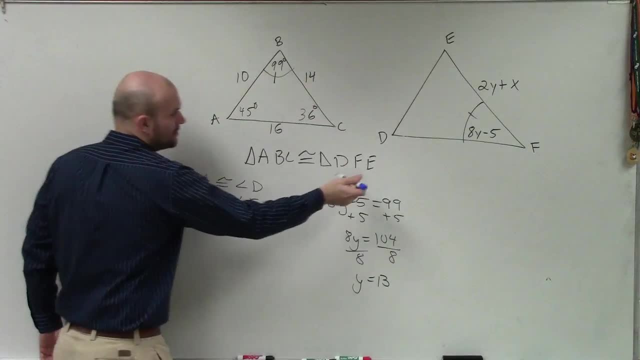 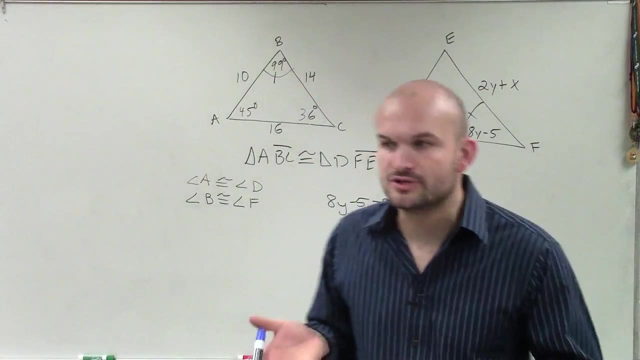 Fe. this line, Fe, is congruent to Bc. OK, So when you guys are trying to determine your congruent parts, look at how the triangle is labeled. Don't always just assume by looking at the picture That's where they're going to try to trick you. 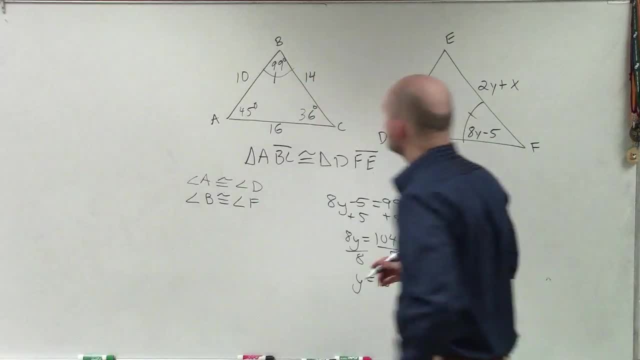 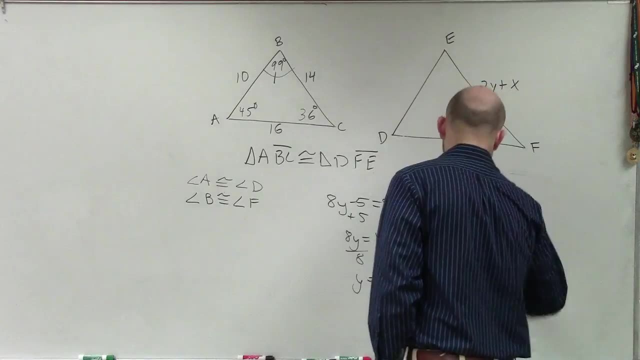 and that's where you're going to make the mistake. So if Fe is congruent to Bc, then I can say that 2y plus x is equal, or sorry, let's write it down like this: Fe is congruent to Bc. 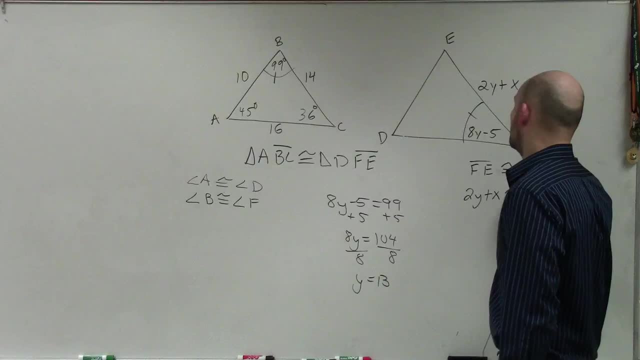 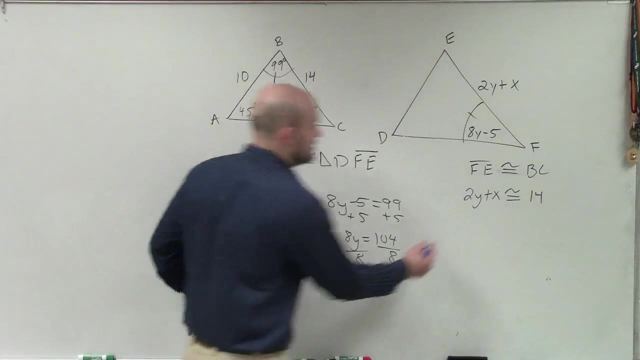 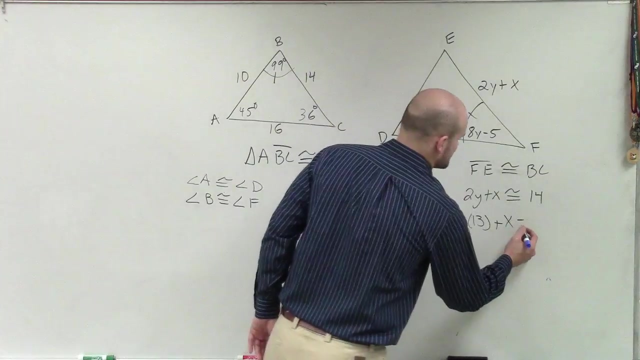 So therefore I can say: 2y plus x is congruent to 14.. Now we know what y is, though correct, So we got y. So I can now say: 2 times 13 plus x. Well, 2 times 13 is going to equal is: 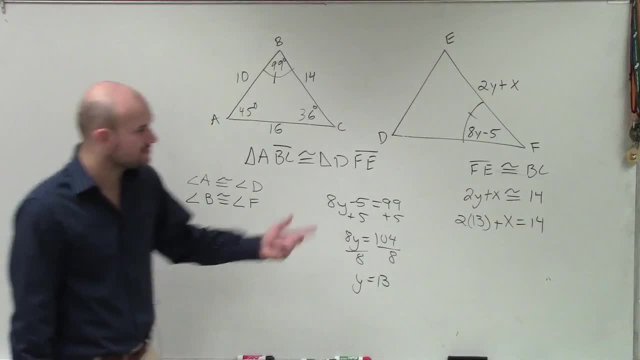 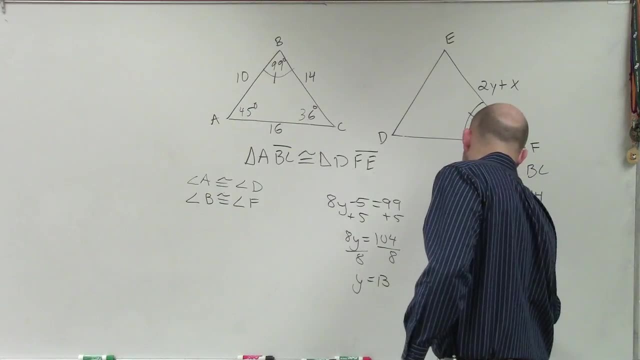 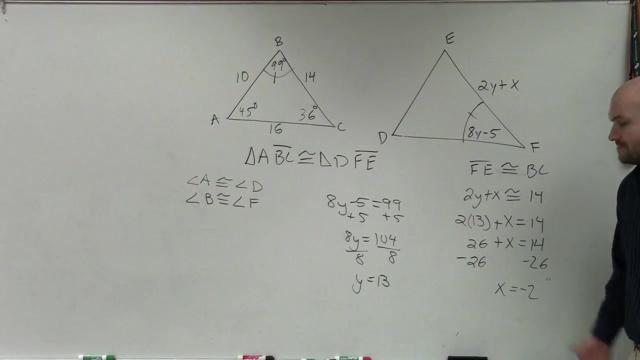 now I'm just going to solve them. I'm not going to use congruency, I'm just going to use the equal sign to solve. So 2 times 13 is going to be 26 plus x equals 14,, minus 26,, minus 26,. x equals negative 2, OK.